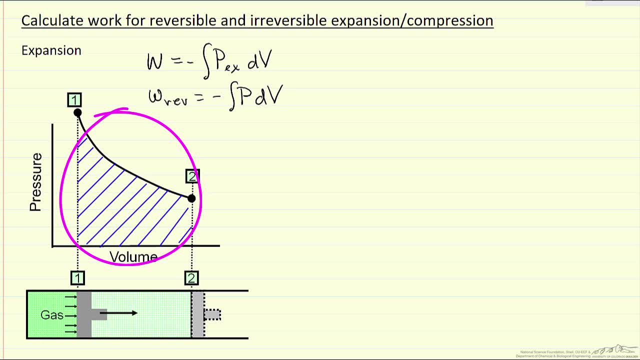 pressure of the gas. That means the work is the area under the curve shown here cross-hatched. This is reversible work. The area is proportional to the reversible work As we expand from point one to point two and the piston then moves from left to right. So now let's look. 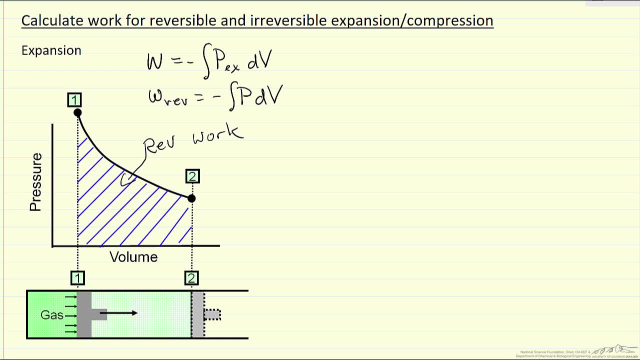 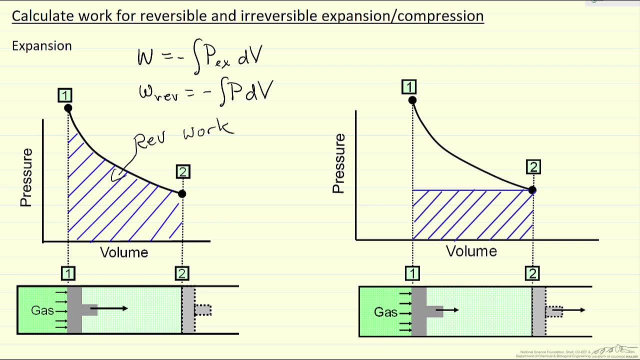 in contrast to an irreversible process. So I am showing a specific irreversible process and there is essentially an infinite number. but here we are going to expand where the final pressure is pressure two. Again, work is equal to p external dv. I am making the external pressure of the final pressure so p external delta V In this area. now this: 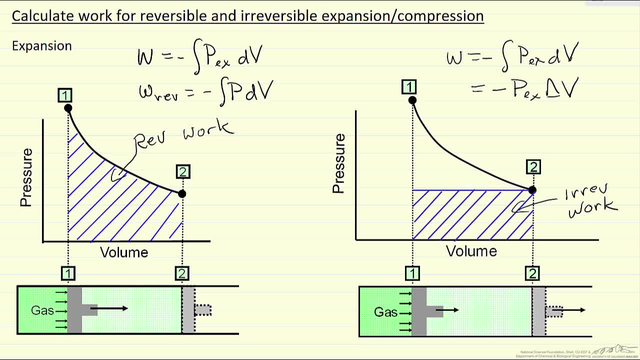 is the irreversible work. S y, Lauren D, A, Q. the irreversible work is smaller. so this is work, irreversible. The work is smaller, we have less resisting force. This, of course, is only one of many ways we could carry out an irreversible process. 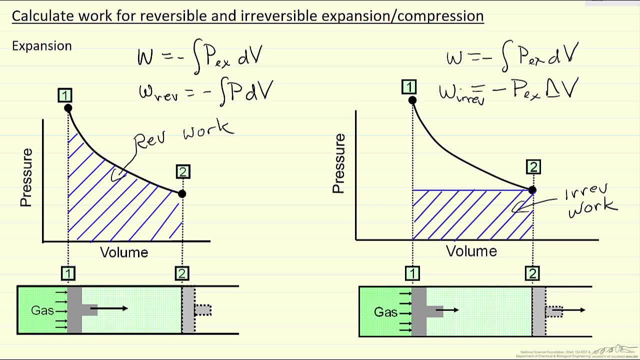 We could do it in steps, where we might first go to half the pressure and get an area, for example, like this, and then get a second area here for the other half, or we could have no resistance, get no work out when we do an irreversible expansion. 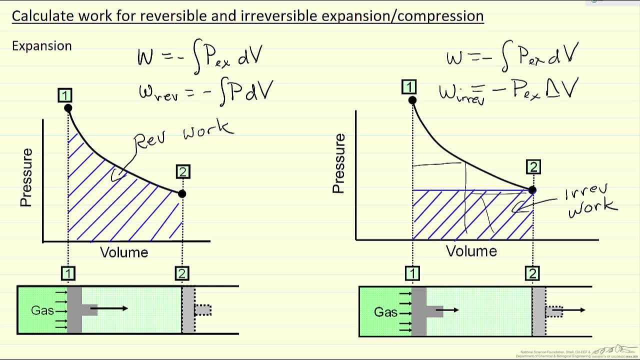 But when we're doing expansion, the irreversible work's gonna be less than the reversible work And these two processes are for any pathway. it doesn't have to be adiabatic or isothermal, can be something in between, for example. 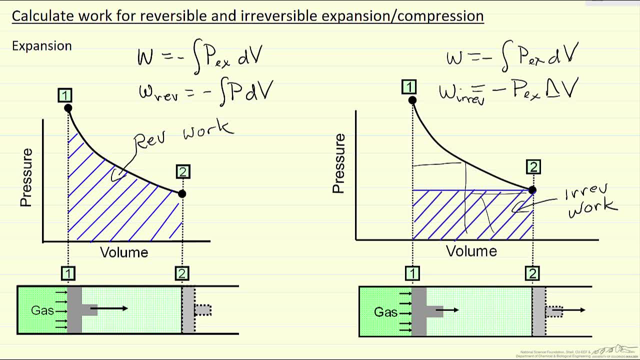 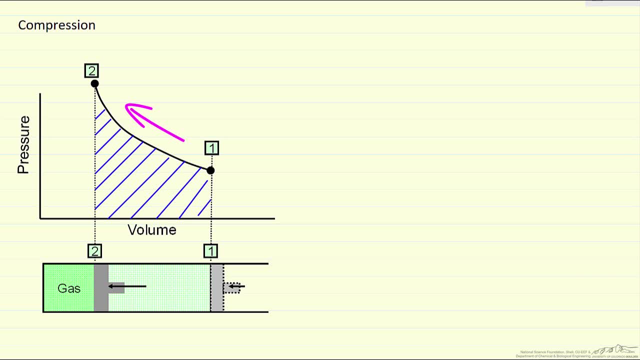 So this expansion? let's look at the case now for compression. So of course, for compression we're gonna start at the low pressure- 0.1, and go to the higher pressure Again. work is for a reversible process. 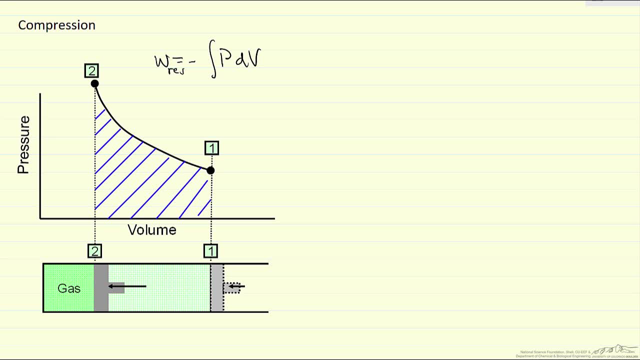 integral of the pressure to gas dv with a minus sign, And so this again reversible work looks identical, but the sign's gonna be opposite for the numerical value. we're putting work into the system to compress it as the gas moves from a larger volume to the smaller volume.